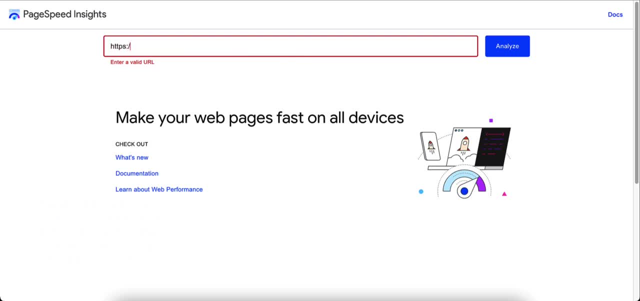 So I'm going to put in my website here, which is tennisdailyxyz, and then we'll hit And the tool is going to go ahead and analyze for mobile. The reason why I analyze for mobile is because most people are going to your site on mobile nowadays. 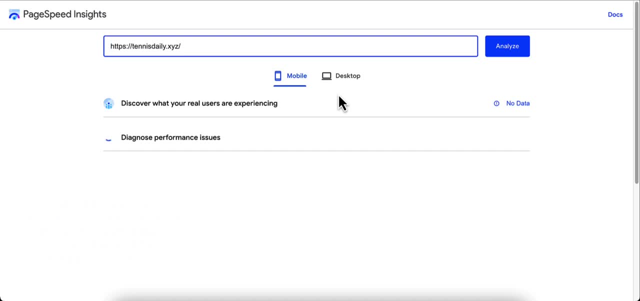 and that number is just going to continue to rise. So what it's doing is it's going to discover what your real users are experiencing. It's diagnosing performance issues, and this might take a couple minutes to do, so I'm going to go ahead and do that. 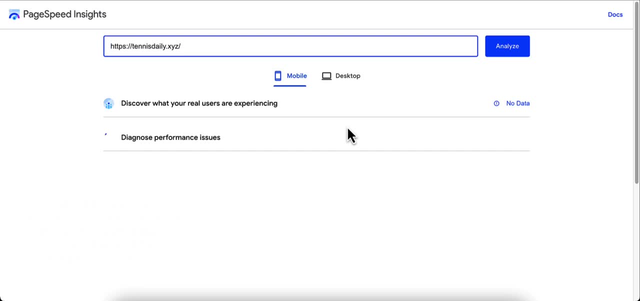 So I'm going to go ahead and do that. So I'm going to go ahead and pause the video while it's doing its thing and I'll be right back when it's finished. All right, so this is my Google PageSpeed Insight score. 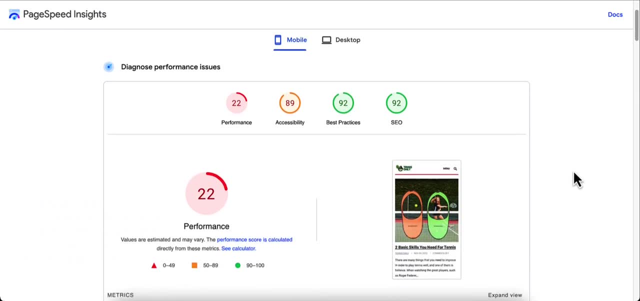 It's absolutely terrible. It's 22.. It's horrible. That's horrible. So we're going to go ahead and optimize this. Now, what you will see could be different from my optimization because of your web host. If I have a faster web host than you, mine could be more. 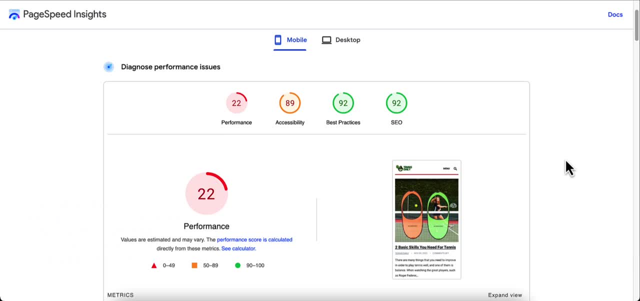 or yours could be more, depending on the web hosting that you have. I have a dedicated Hostinger server, so mine will hopefully be fast once this is finished. If you have shared web hosting, then yours may not be as fast as mine. I'll drop a link down below to the. 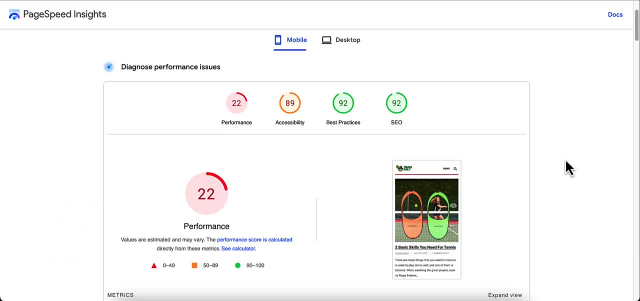 Hostinger dedicated IP that I have and to that plan. that way, you can see, Now Black Friday is right around the corner, so you might be able to score some deals on that as well. So let's go over. I'm going to keep this up so we can come back to it. 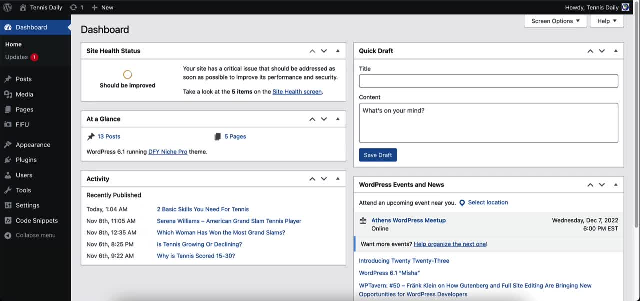 and we're going to go over to my website here, Log into your WordPress dashboard and from our WordPress dashboard, we're going to go ahead and install a plugin. So we're going to go to Plugins. hover over Plugins. hover over on the left-hand side of the screen and click Add New. 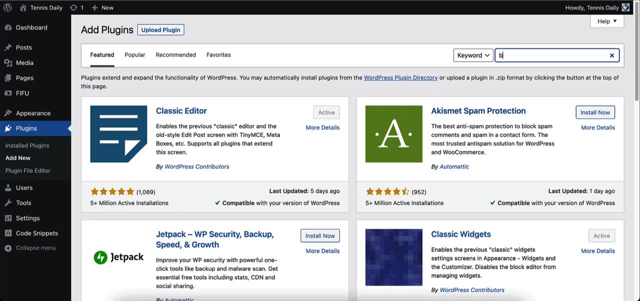 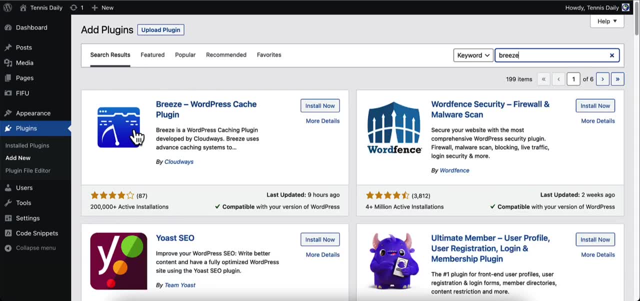 And then we're going to search for a plugin called Breeze B-R-E-E-Z-E And it's going to pull up this plugin right here. It should be the very first one. Breeze WordPress Cache Plugin by Cloudways. Go ahead and install that by clicking on the Install button. 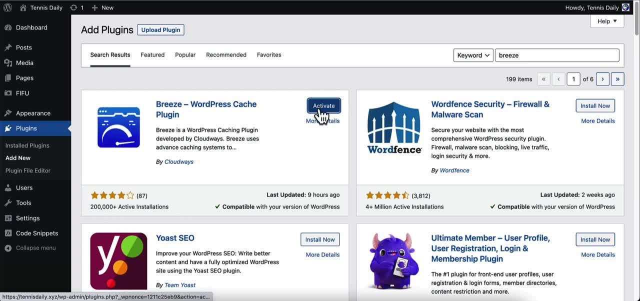 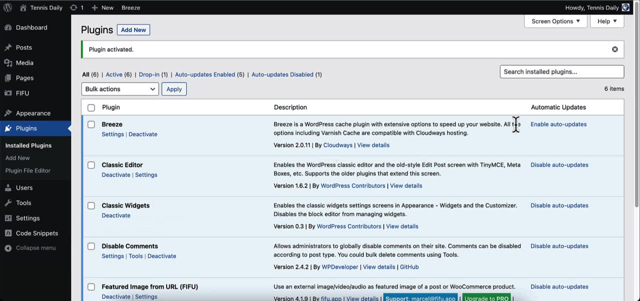 and then we'll click on the Activate button when that pops up. So that has been, That has been activated. and then always, what I always do is click on the Enable Auto Updates over here on the right-hand side to make sure that everything is auto-updated. 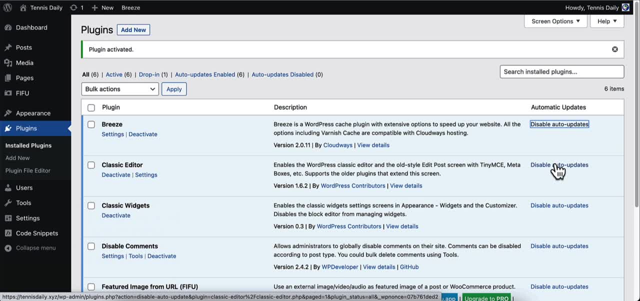 That way, you get all of the security, the latest security features as well. So now we have Breeze installed, We can either click on Settings right here or you can go hover over Settings in Breeze, because this is where you're going to find it if you're ever going to need. 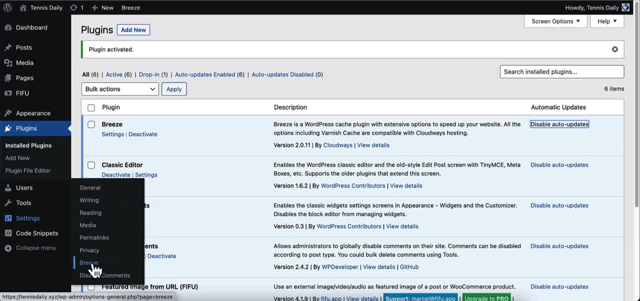 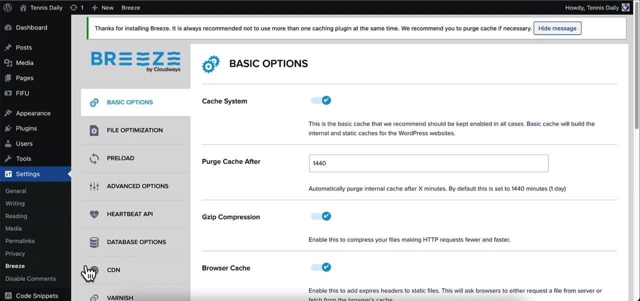 to make any changes to it later on. So Settings: hover over Settings and click on Breeze and here are our options. So, like I said, I'm going to try to go slow because there are some optimizations that we need to do within this plugin. 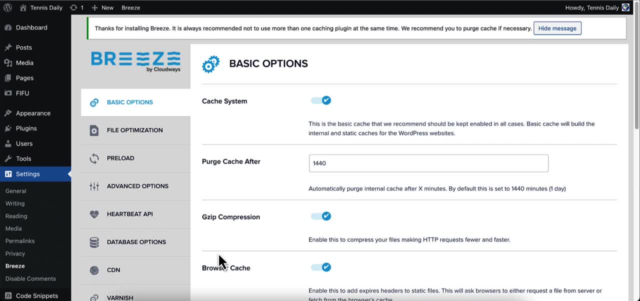 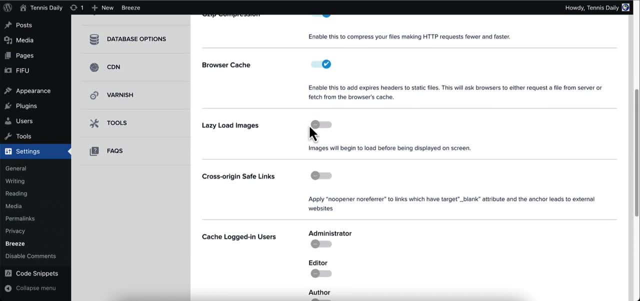 So we're going to go here and we're going to start here at Basic Options, and we want to scroll down here and we want to turn on Lazy Load, Images and Iframe Lazy Load and we want to Enable Native Browser. Lazy Load. 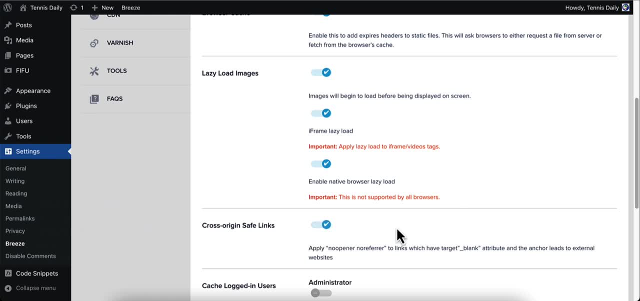 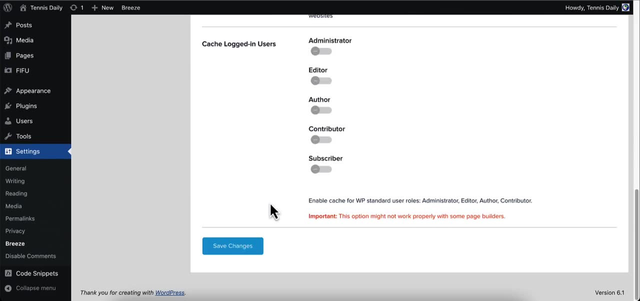 and we want to Enable Cross-Origin Safe Links, And I believe, yep, that's all we need to do with that. Now, when we do these, just make sure you hit Save Changes at the bottom before we go over to another tab, because it will not save. 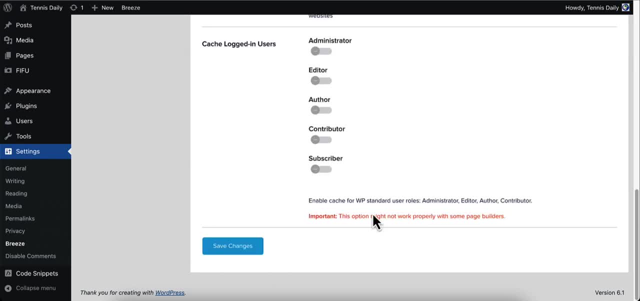 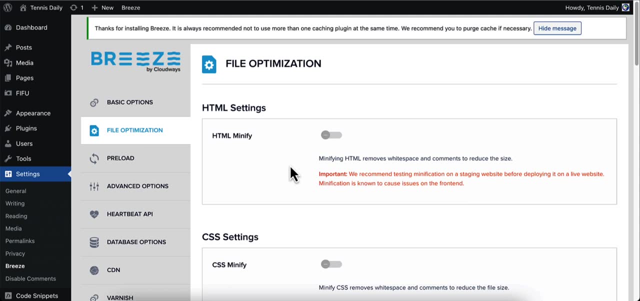 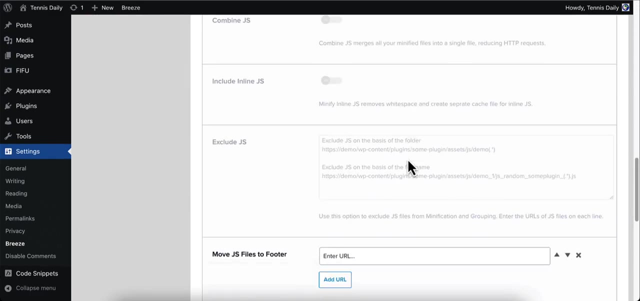 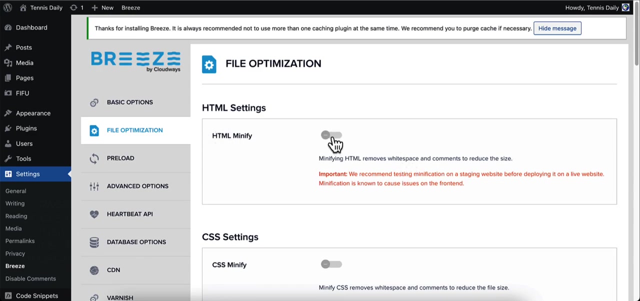 So make sure you hit Save, Scroll down and hit Save Changes. Okay, the changes have been saved. Now we're going to go over to File Optimization and we're going to need to scroll down here and we need to do HTML Minify and we need to do: 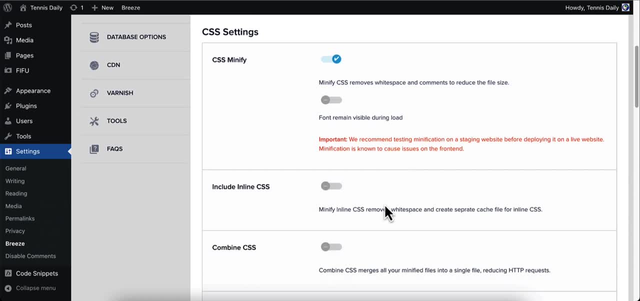 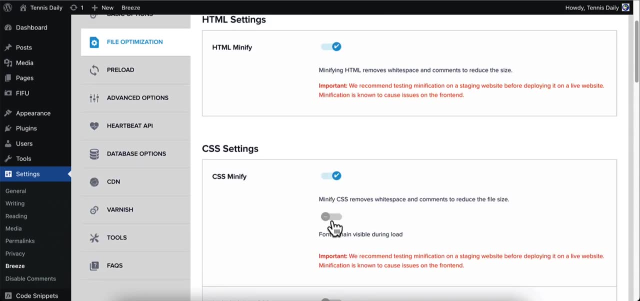 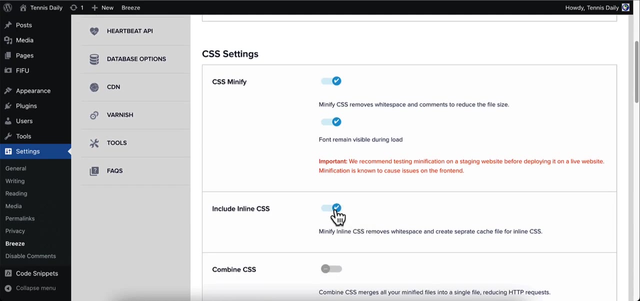 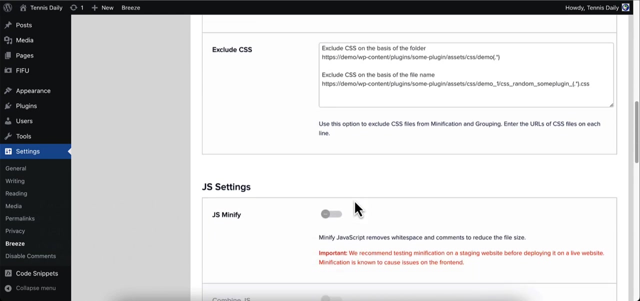 we need to enable CSS Minify, Okay, And we need to do Font Remain Visible During Load. We need to enable Include Inline CSS. We need to enable Combined CSS: Scroll down a little bit and then we're going to enable JS Minify, which is JavaScript. 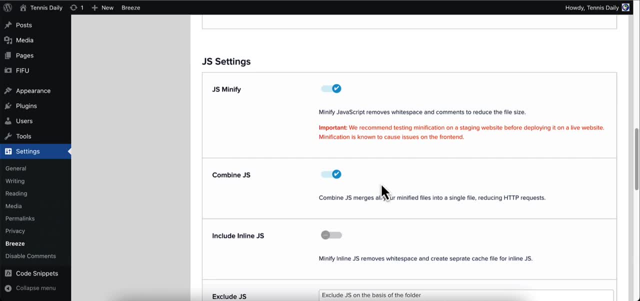 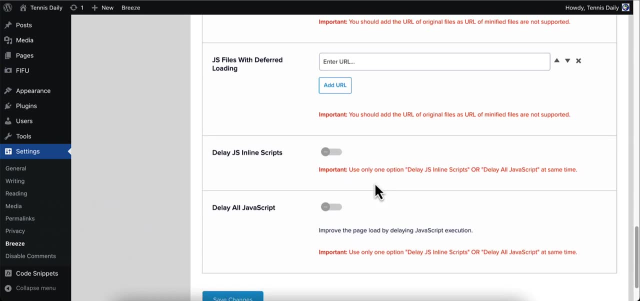 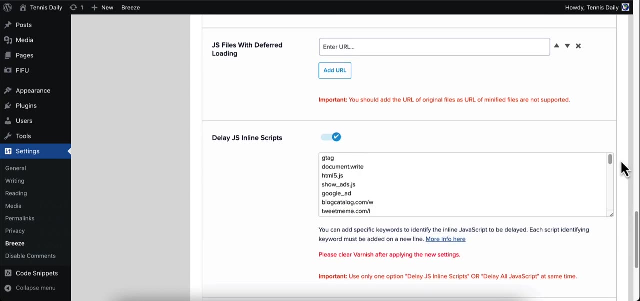 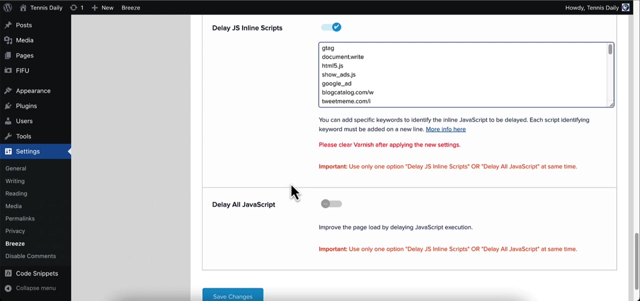 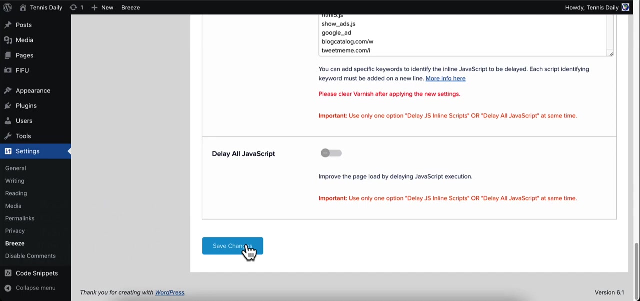 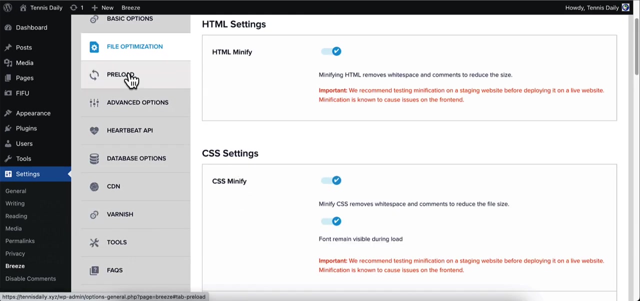 We're going to enable Combine JavaScript And we're going to do Delay JavaScript Inline Scripts. Keep everything here the same. Don't change anything in this box And hit Save Changes at the bottom. Okay, now that our changes are saved here, scroll back up and go to Preload tab at the left-hand side. 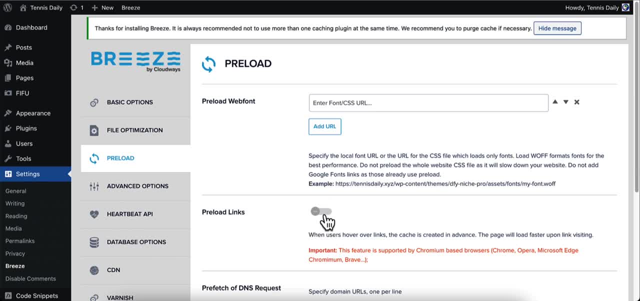 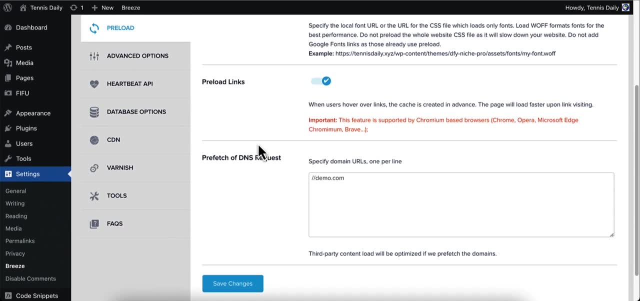 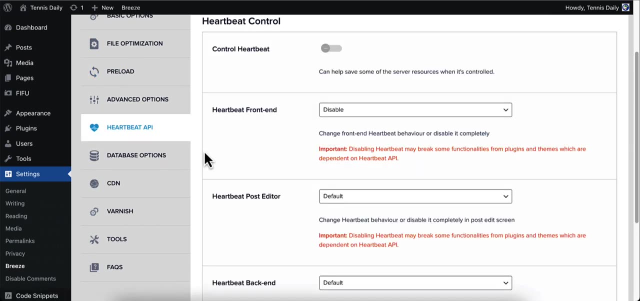 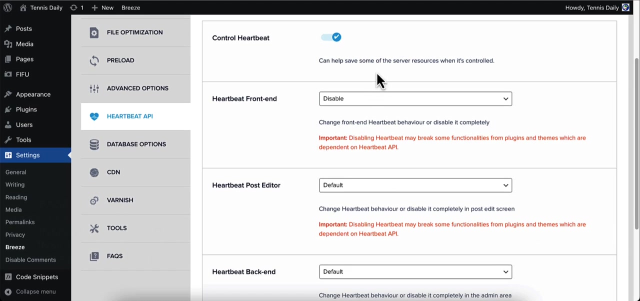 If, then we want to enable this option that says Preload Links. enable that Scroll down. Save Then under Heartbeat API, this tab here at the side, click on that. We want to enable Control Heartbeat And we want to set our heartbeat front end to every five minutes. 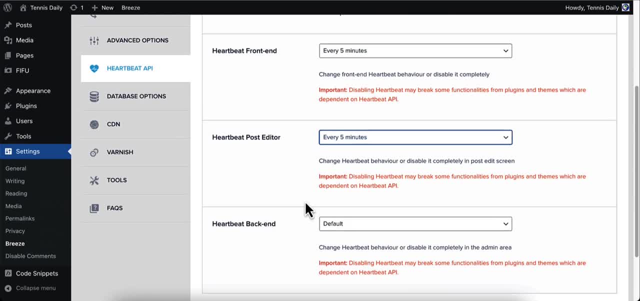 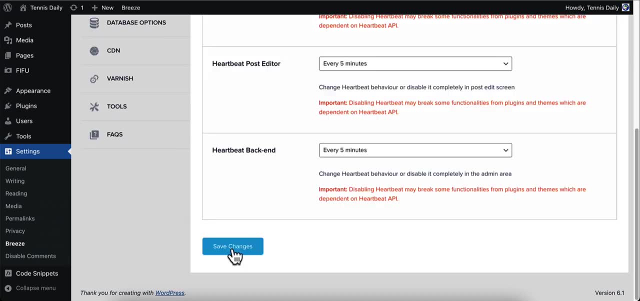 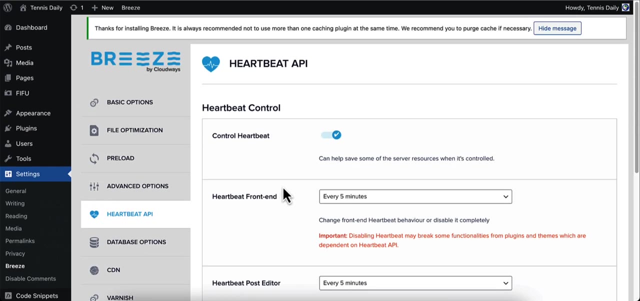 We want to do that here as well. Heartbeat Post Editor to every five minutes And the heartbeat back end to every five minutes And hit Save Changes. Okay, that's it. That's all that we need to change under Breeze. 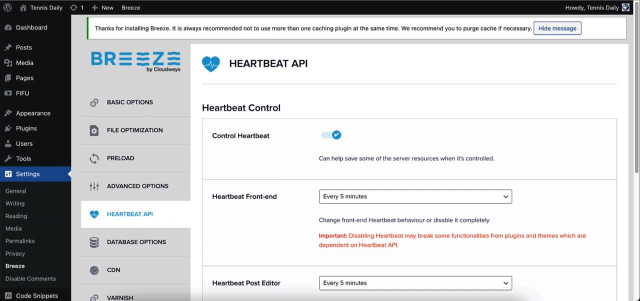 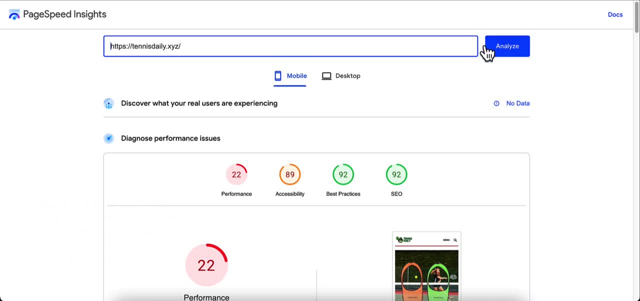 So, now that all of that has been changed, let's go ahead back to our PageSpeed Insights And let's go ahead and run this thing again. So click Analyze at the top. Now it's going to go through its thing: Diagnosing Performance Issues. 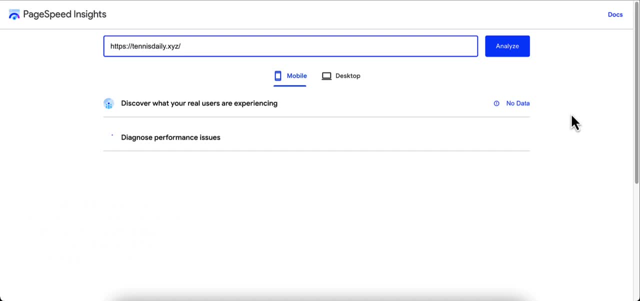 And, once again, I'm going to pause the video And once it's finished I will be back. All right, So now it's done. All right, So now it's done. All right, All right, All right, It's finished.